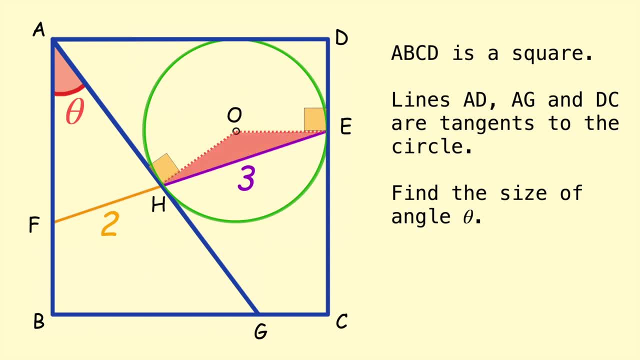 tangents is 90 degrees. Also, the base angles of that triangle are equal. So we have two equal angles here, I've marked in green. Also, these two angles over here are going to be equal: BFH and FHG. FHG is vertically opposite, BFH is alternate. So all of those four angles I've marked in green. 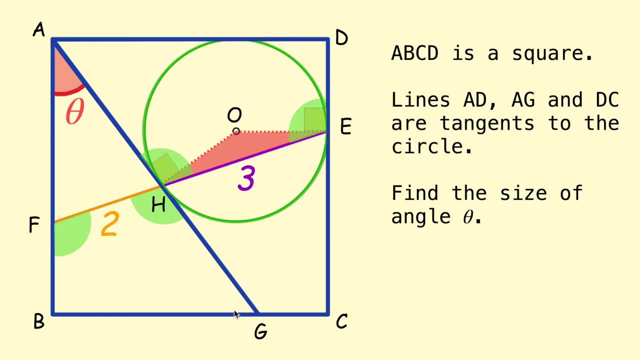 are equal Now, because AB and AG are straight lines, then these two base angles of this triangle AFH will also be equal. So we have an isosceles triangle AFH that tells us AF equals AH and also AI equals AH because they're tangents to a point. That's one of the other circle theorems we're going to be. 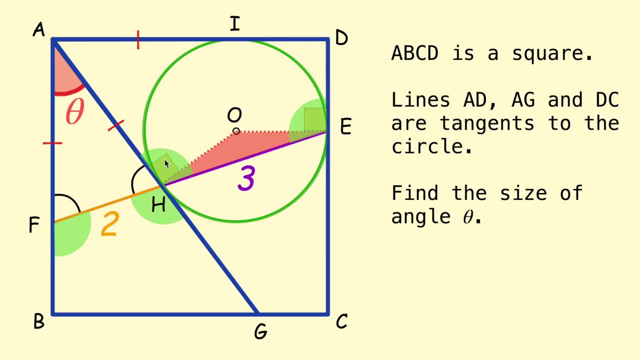 using here. So so far we've used two circle theorems: the angle between a radius and a tangent, and tangents to a point. If you want to know more about all the circle theorems you need to know for GCSE mathematics. 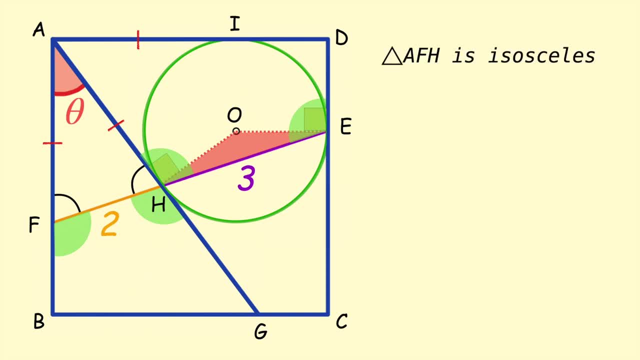 check out my video on those. Okay, let's write down what we've found so far. So AFH is isosceles, AF equals AH, equals AI angle, AHE equals DEH, And also we know that the base angles of this 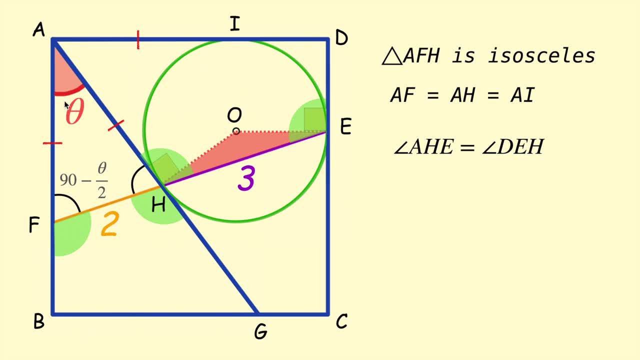 triangle will be 90. take theta on two. Think about the angles in a triangle. they add up to 180 degrees. So these two angles added together will be 180 degrees. So we know that the base angles of this triangle will be 90. take theta on two, So these two angles added together will be 180 degrees. 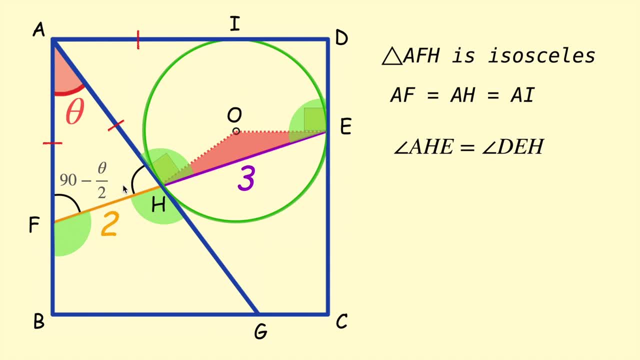 Yeah, 80. take theta And then, to find them individually, divide by two. So that's 90, take theta on two. Then this green angle is the external angle of this triangle. To find that you can add these two angles together, theta plus 90, take theta on two. So the green angle is 90, take theta on two plus. 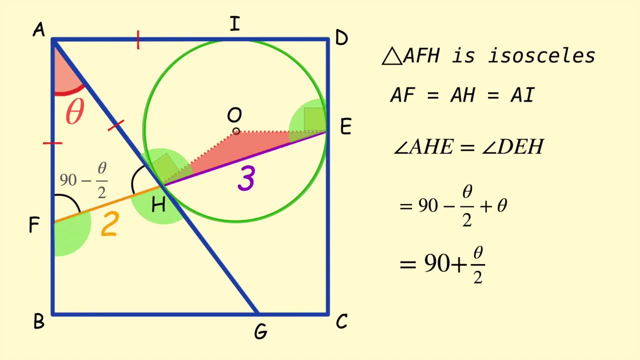 theta or 90 plus theta on two. okay, that tells us that that angle in there, the base angle of that isosceles triangle, must be theta on two. Kann't figure out if that's an angle that's coming from the left triangle. of that angle must be theta on two. Can you see that Makes sense to music? I suppose not ownership triangle. Well, that does what it's actually saying. you could kind ofidden out of that. Do we use an angle of that Rodriguez triangle? the base angle of that ISOceles triangle must be theta on two, right that's. 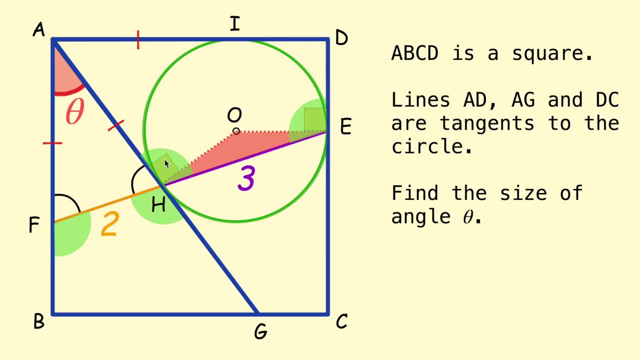 using here. So so far we've used two circle theorems: the angle between a radius and a tangent, and tangents to a point. If you want to know more about all the circle theorems you need to know for GCSE mathematics. 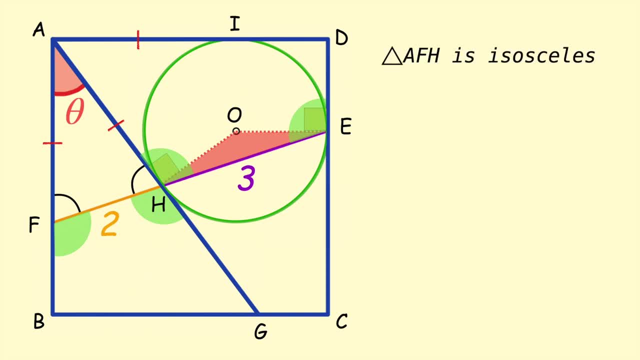 check out my video on those. Okay, let's write down what we've found so far. So AFH is isosceles, AF equals AH, equals AI angle, AHE equals DEH, And also we know that the base angles of this 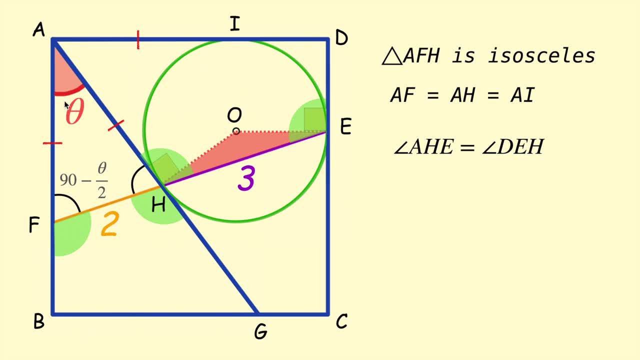 triangle will be 90. take theta on two. Think about the angles in a triangle. they add up to 180 degrees. So these two angles added together will be 180 degrees. So we know that the base angles of this triangle will be 90. take theta on two, So these two angles added together will be 180 degrees. 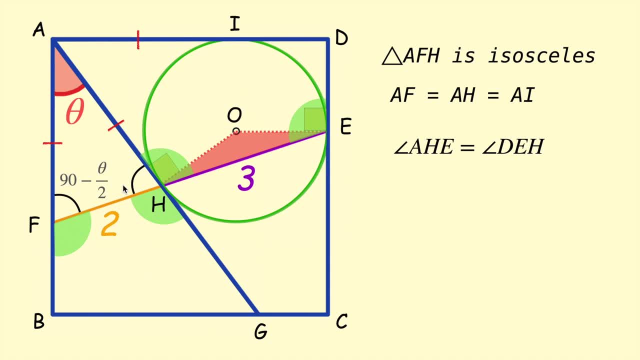 So we know that the base angles are 90 ace theta, and then minus 90, take theta, plus 180, take theta and then, to find them individually, divide by two, so that's 90, Take theta on two. Then this green angle is the external angle of this triangle. To find that you can add these two. 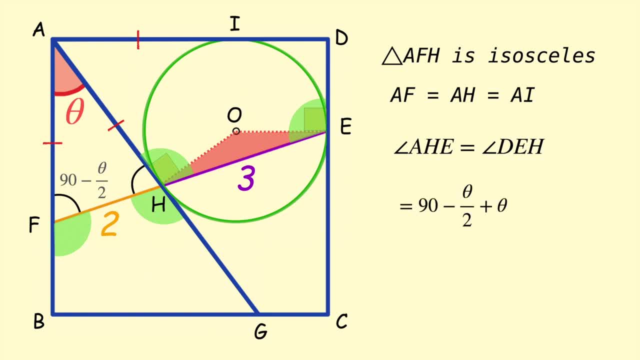 angles together: theta plus 90. take theta on two. So the green angle is 90. take theta on two plus theta, or 90 plus theta on two. Okay, that tells us that that angle in there, the base angle of that isosceles triangle, must be theta on two right. Then we also need to calculate it, We need to. 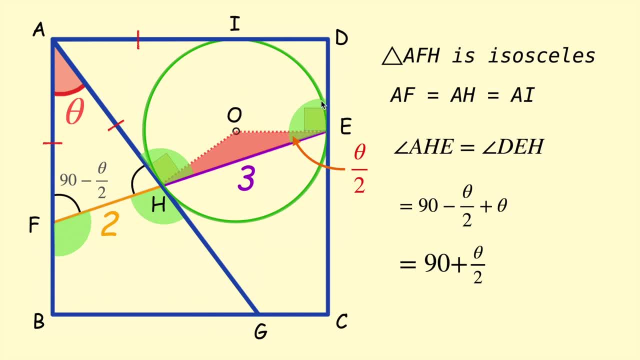 on 2, right, The entire angle is 90 plus theta on 2.. This part's 90, this part's theta on 2.. Also, note that ID is equal to the radius of the circle, which is also equal to FB, because 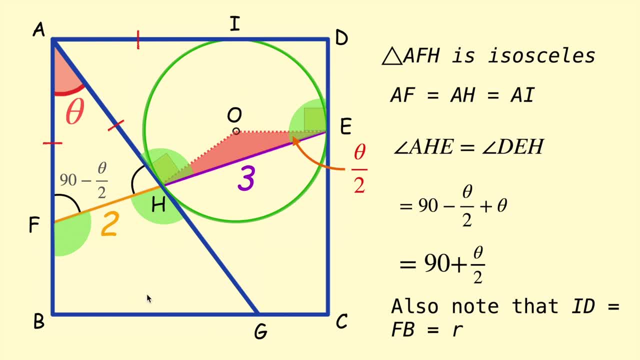 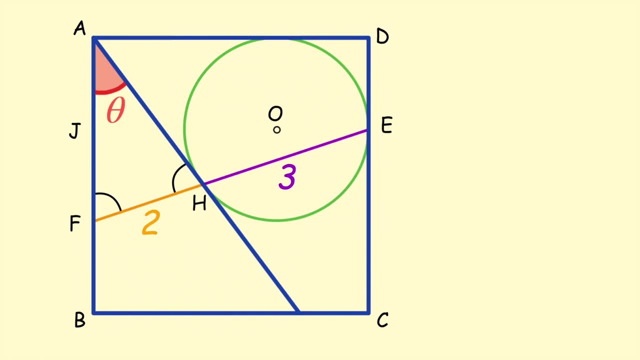 AF and AI are equal, so ID equals FB, which equals R, the radius. Okay, so we're going to use all that information now and draw some similar right triangles. The first right triangle I'm going to draw is EJF, so I'm drawing a horizontal line from E to J through the 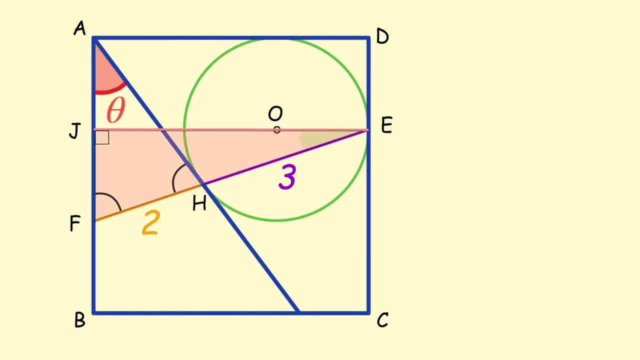 centre of the circle. and this right triangle, as we just showed, has an angle of theta on 2.. Next we're going to draw another right triangle, bisecting the isosceles triangle, that also has an angle of theta on 2.. And also we know the short leg of that right triangle. 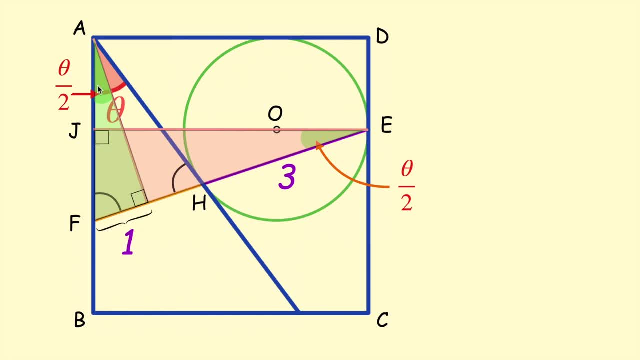 will be 1, again because we've bisected that isosceles triangle. We cut the angle in half and we cut the base in half, so in relation to the other lengths, this length is equal one and the other right triangle we're going to create is inside the circle. 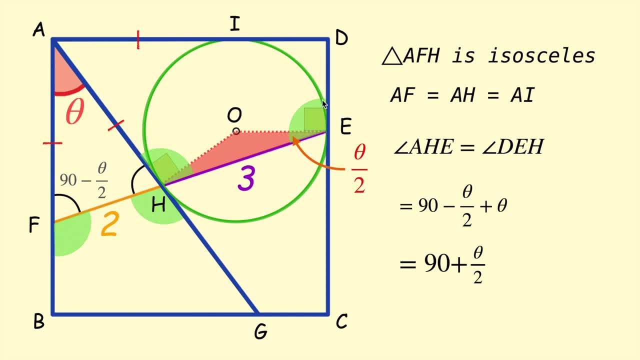 the entire angle is 90, plus theta on 2.. This part's 90, this part's theta on 2.. Also, note that ID is equal to the radius of the circle, which is also equal to FB, because AF and AI are equal. so ID equals FB, which equals R, the radius. Okay, so we're going to use all that. 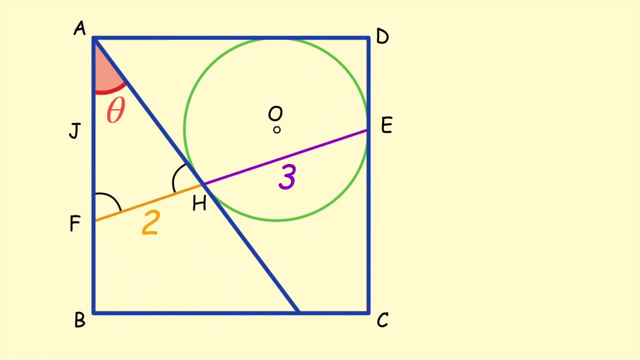 information now and draw some similar right triangles. The first right triangle I'm going to draw is EJF, so I'm drawing a horizontal line from E to J through the center of the circle and this right triangle, as we just showed, has an angle of theta on 2.. Next we're going to draw 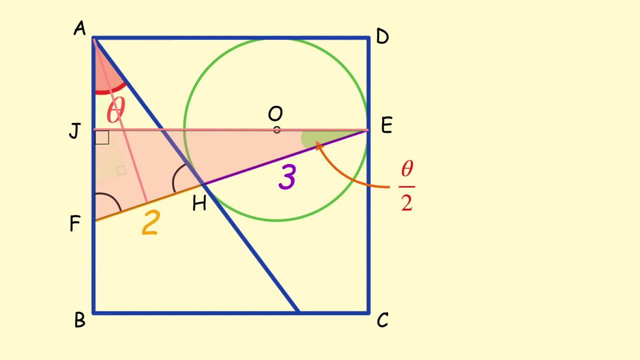 another right triangle, bisecting the isosceles triangle, That also has an angle of theta on 2, and also we know the short leg of that right triangle will be 1.. Again, because we bisected that isosceles triangle, we cut the angle in half and we cut the base in half. so, in relation to the 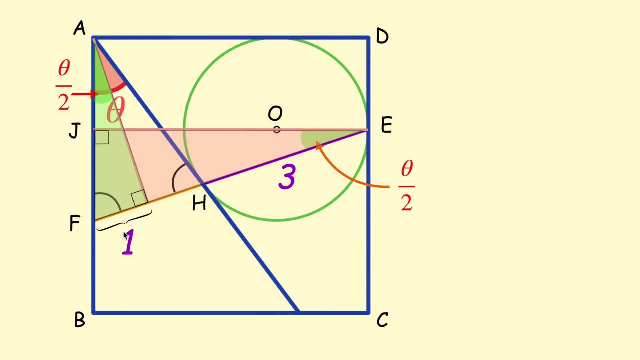 other lengths. this length is 1. And the other right triangle we're going to create is inside the circle here, Inside the semicircle that also has an angle of theta on 2. Because all of the angles are the same, we've created three. 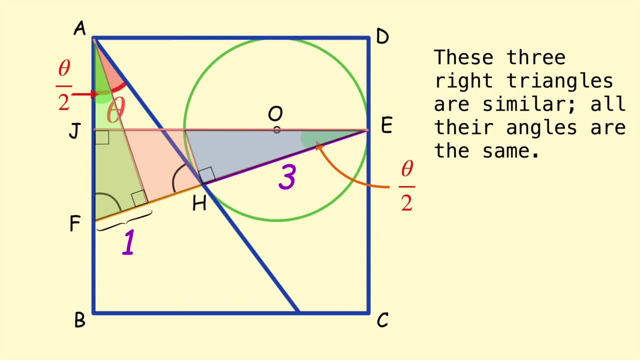 similar right triangles. A few other things to note. we'll let JF equal A, so we're going to let this length here equal A. So then AF equals R plus A, so AJ is R, so AF is R plus A. 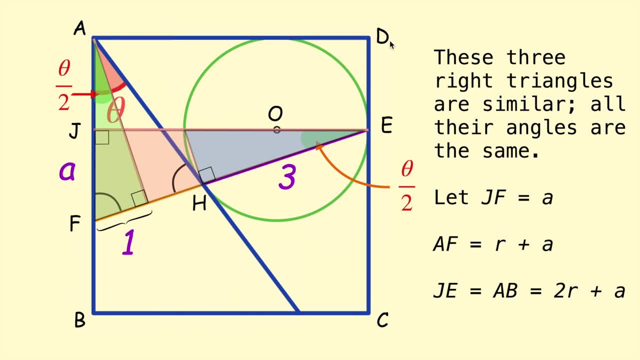 Also JE, which is the same as the length side length of the square. that's equal to AB, which is equal to 2R plus A. Okay, so let's look at these three right triangles separately. now We know the. 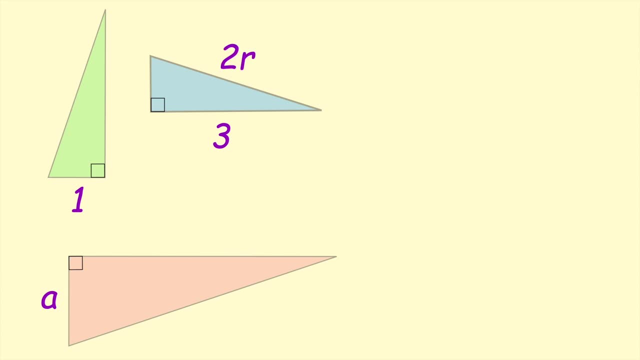 hypotenuse of the blue right triangle is 2R, 2 times the radius of the circle. We know the hypotenuse of the green right triangle is R plus A and we know the hypotenuse of the red right triangle was 5 in relation to the other lengths. Next, we know the long leg. 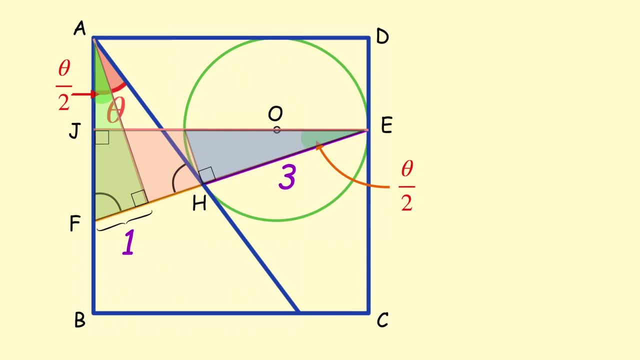 here inside the semicircle that also has an angle of theta on two, because of all of the angles are the same. we've created three similar right triangles. a few other things to note. we'll let JF equal a, so we're going to let this length here. 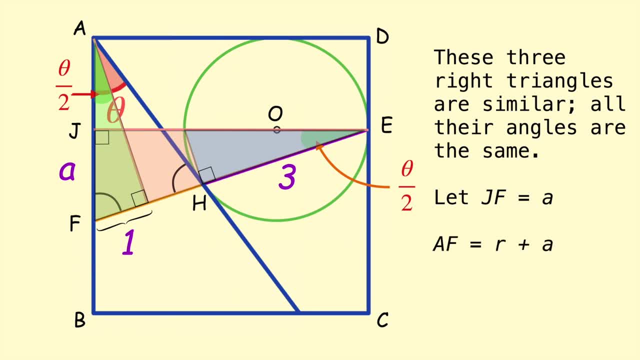 equal a. so then a F equals R plus a, so a J is R, so a F is R plus a. also J, E, which is the same as the length, side length of the square. that's equal to a B, which is equal to 2 R plus a. okay, so let's look at these three right triangles. 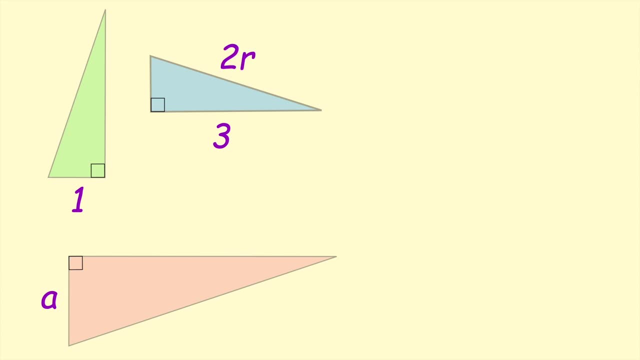 separately. now we know the hypotenuse of the blue right triangle is 2 R 2 times the radius of the circle. we know the hypotenuse of the triangle is 2 R 2 times the radius of the circle. we know the hypotenuse of the 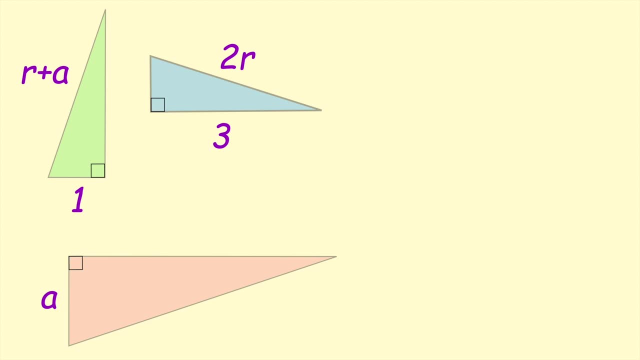 green right triangle is R plus a, and we know the hypotenuse of the red right triangle was 5 in relation to the other lengths. next, we know the long leg of the large right triangle is 2 R plus a. so using similar triangles we can compare. 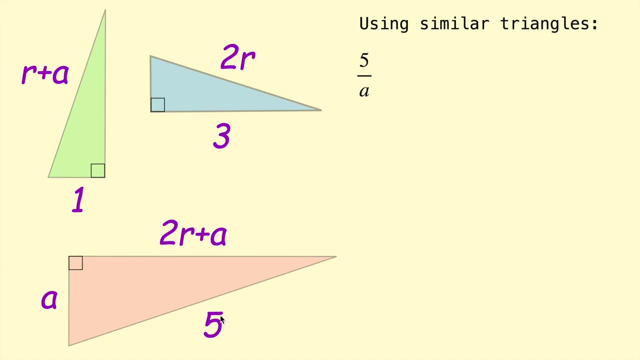 the ratios of the sides of those triangles. so the ratio of the hypotenuse to the short leg on this triangle, 5 to a, will equal this, the same ratio on the green right triangle. so 5 on a is equal to R plus a to 1. this equation allows us to write R in terms of a. so 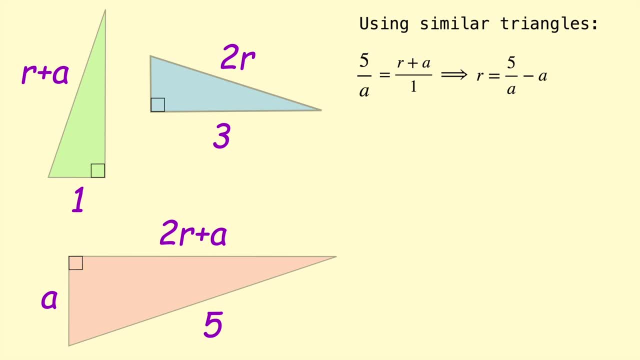 rearranging. we can say: R equals 5 on a take a, and we can also write that as 5 take a squared on a. next, we can create another equation using the other ratios. so 2 R plus a to 5 is the long leg to the hypotenuse, so that ratio is equal. 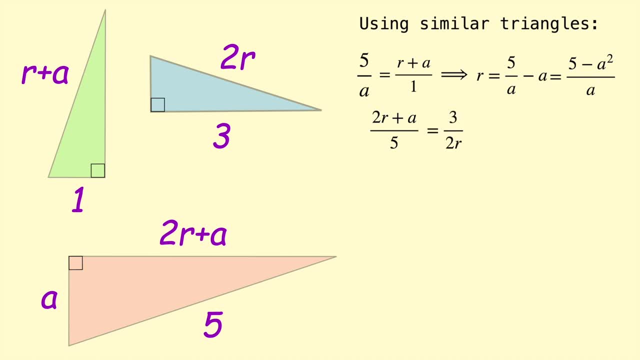 to the same ratio on the blue triangle, 3 to 2 R, and these two equations are actually enough to solve for a and R. so, rearranging this, we get 4 R squared plus 2 R, 2 RA equal to 15. so I multiplied this. 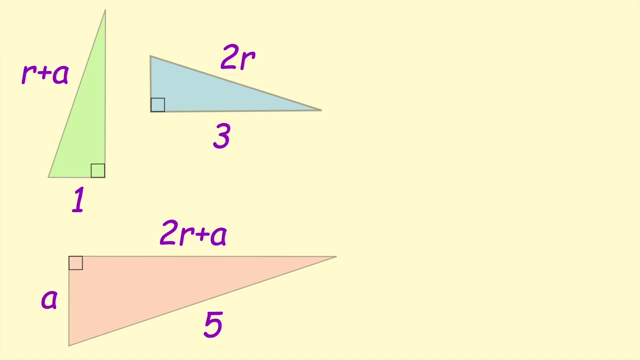 of the large right triangle is 2R plus A. So using similar triangles we can compare the ratios of the sides of those triangles. So the ratio of the hypotenuse to the short leg on this triangle, 5 to A, will equal the same ratio on the green right triangle. So 5 on A is equal to R plus A. 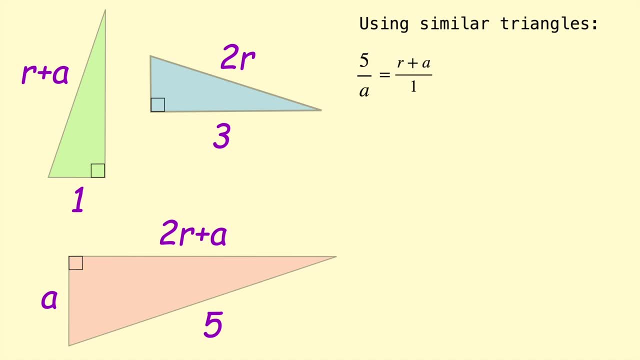 to 1.. This equation allows us to write R in terms of A, So rearranging, we can say: R equals 5 on A take A, And we can also write that as 5 take A squared on A. Next, we can create another. 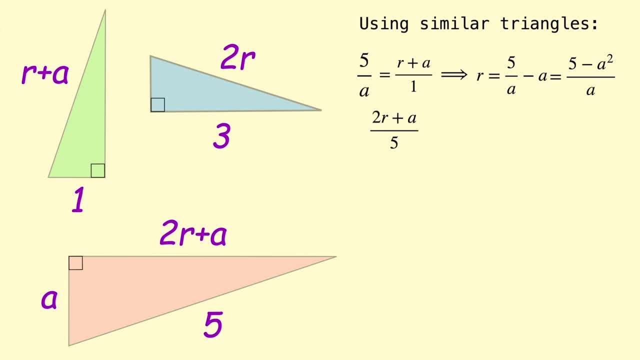 equation using the other ratios. So 2R plus A to 5 is the long leg to the hypotenuse. So that ratio is equal to the same ratio on the blue triangle 3 to 2R, And these two equations are actually. 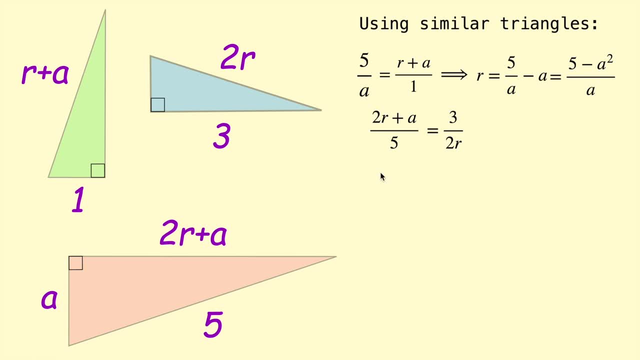 enough to solve for A and R. So, rearranging this, we get 4R squared, 2R squared, 2R squared squared plus 2R, 2RA, equal to 15.. So I multiplied this R by 2R, this R by 5.. And now, because we have 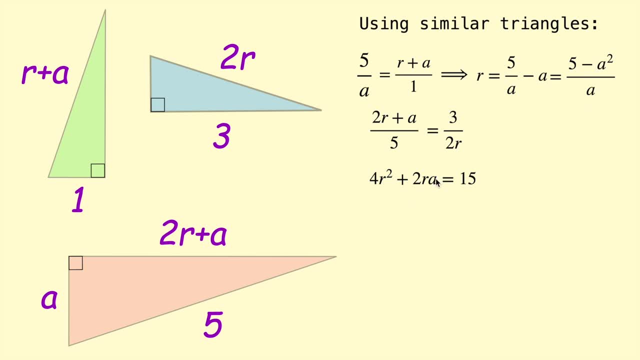 R in terms of A. we can substitute that in for R here and then solve for A. So we're going to take that value for R, substitute that into that equation. The algebra is a bit messy. Going to have to spend some time simplifying that because this is a fraction. So do all of that simplifying. 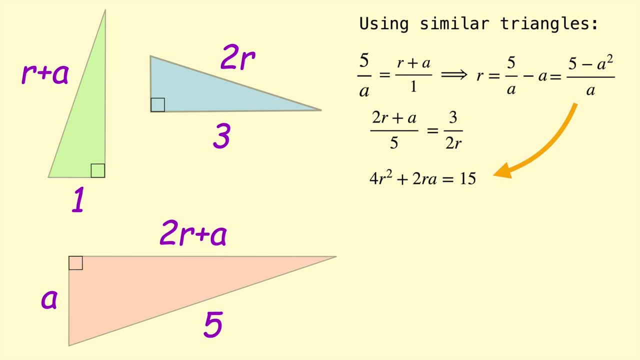 do all of the arranging, rearranging. After all of that, it's a bit of a messy algebra. You should get this equation: 2A to the power 4: take 45A squared plus 100 equals 0. And this is basically a quadratic. Well, it's a quartic, but you can. 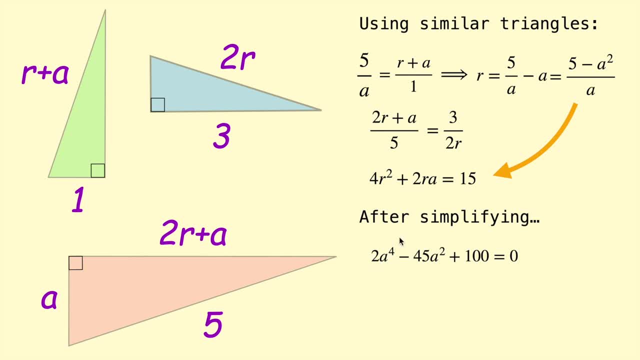 substitute X squared for A to the power 4.. And then it becomes a quadratic that you can solve. You can use the quadratic formula or a quadratic solver, or even possibly factorizing. I don't think I even tried to factorize this. But however you like, you can solve that quadratic. 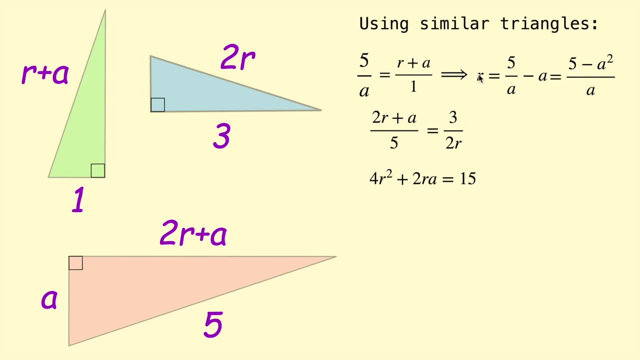 R by 2, R, this R by 5. and now, because we have R in terms of a, we can substitute that in for R here and then solve for a. so we're going to take that value for R, substitute that into that equation- the- the algebra is a bit messy- going to have 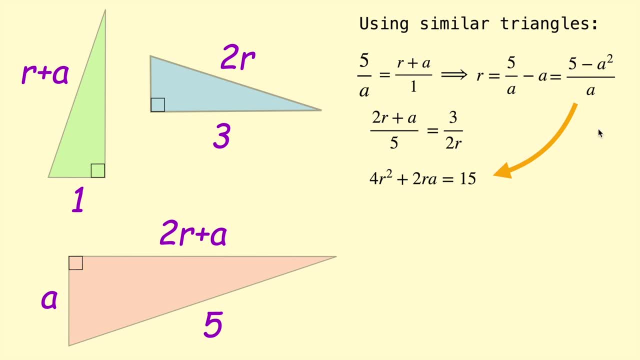 to spend some time simplifying that, because this is a fraction. so do all of that simplifying, do all of the arranging, rearranging after. after all of that- a bit of a messy algebra, you should get this equation: 2 a to the power 4. take 45, a squared plus 100 equals 0 and this is basically a quadratic. 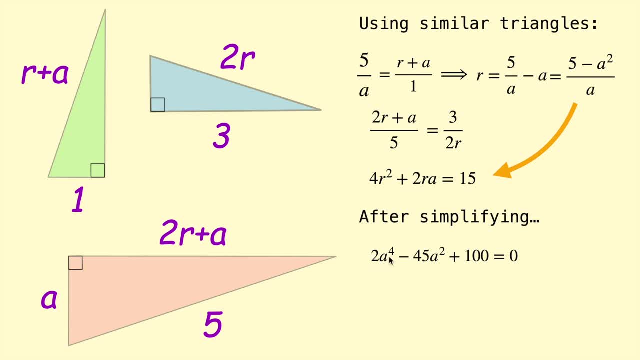 well, it's a quartic, but you can substitute x squared for a to the power 4 and then it becomes a quadratic that you can solve. you can use the quadratic formula or a quadratic solver, or even possibly factorizing. i don't think i even tried to factorize this, but however you like, you can. 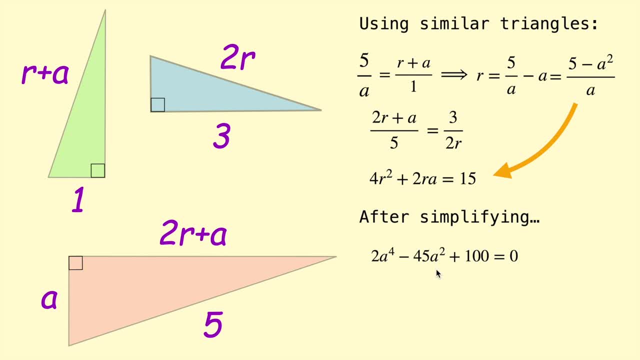 solve that quadratic and you should get two positive solutions. we don't care about the negative solutions because we're talking about lengths. so two positive solutions for a. they are root 10 on 2 and a equals 2 to root 5. one of these we can rule. 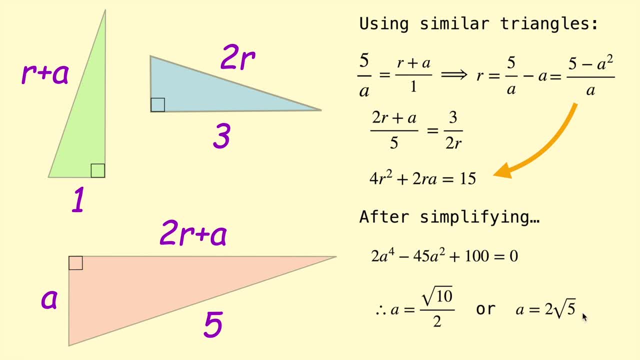 out. we can rule out a and a equals 2 to root 5 and a equals 2 to root 5 and a equals 2 to root 5. to root 5 is about 4.5, which is not possible here if you think about the lengths of these right. 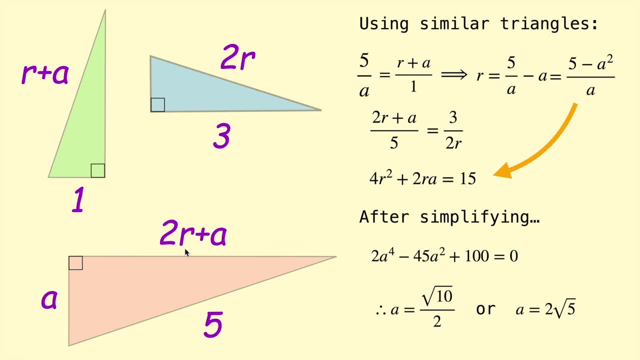 triangles. so, for example, if this length was 4.5, this long leg would be 4.5. it must be less than 5, right? so 2r would have to be less than 1. let's just say so: 2r if 2r is less than 1. 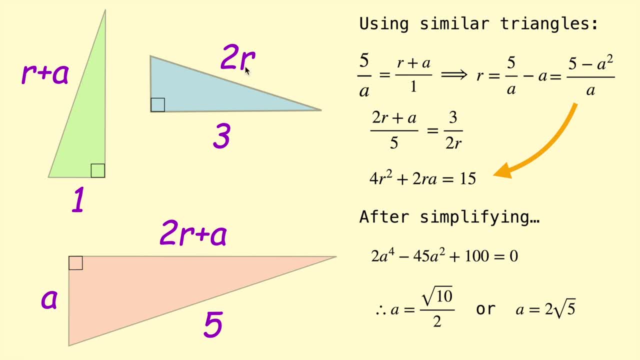 that doesn't fit with this right triangle, because then the hypotenuse would be less than the long leg, which is impossible in a right triangle. okay, so we can rule out 2 root 5 as a possible solution in this case. so we have a solution for a of root 10 on 2, and that's actually. 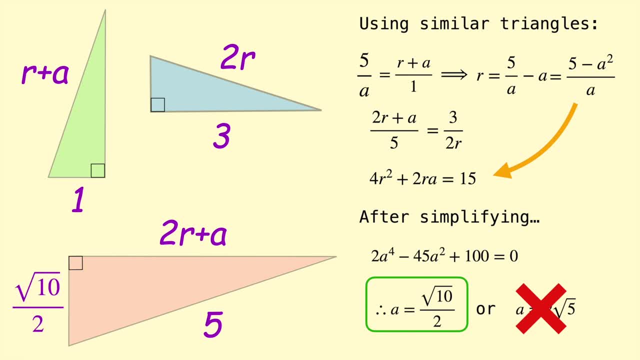 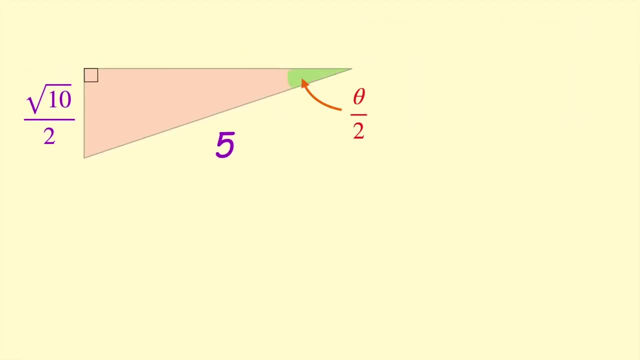 enough to solve for theta. so we now know the side length of this right triangle is root 10 on 2, and remember the angle was theta on 2. so using our trig ratios we can say: sine of theta on 2 equals the opposite side over theta on 2, and that's actually enough to solve for theta on 2. so we can.